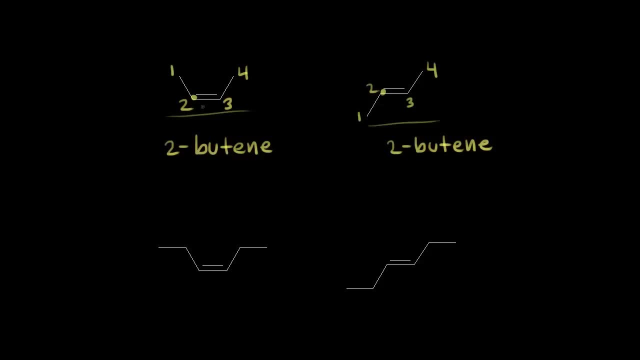 Single bonds have free rotation, but double bonds don't. So you couldn't rotate the molecule on the left to look like a double bond. They look like the molecule on the right. Therefore, they must be isomers of each other And we need a way to distinguish between our isomers. 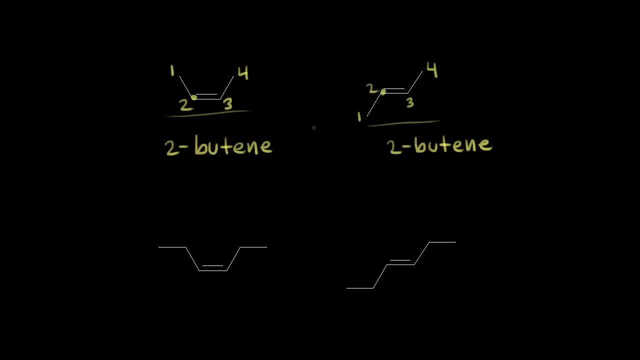 And so one way to do that is to use cis-trans terminology. So if we look at the molecule on the left, we can see we have two methyl groups, And those two methyl groups are on the same side of our double bond. So if I draw a line in here, 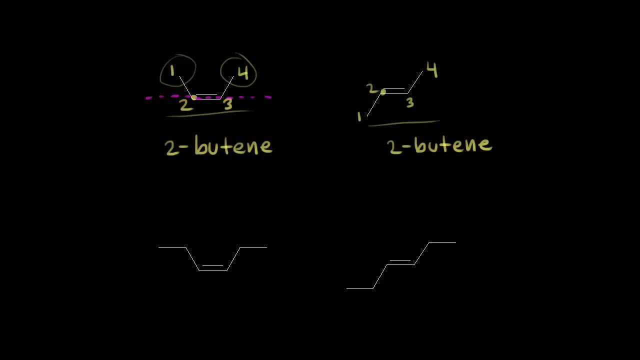 it's easier to see. those two methyl groups are on the same side And we call that the cis isomer, So we put cis in front of our name here. I'm attempting to write it in italics, So this would be cis-2-butene. 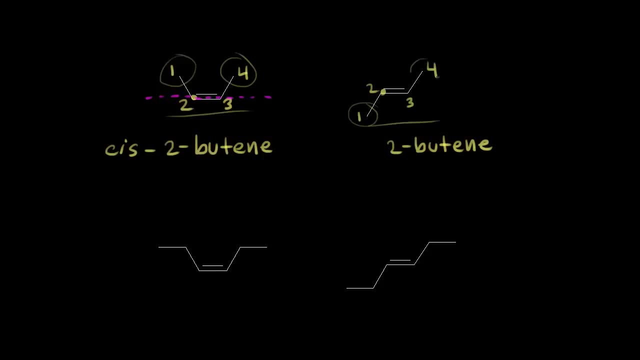 On the right when we look at those methyl groups. these two methyl groups are on opposite sides of the double bond. So I draw a line in here to make it easier to see. those two methyl groups are on opposite sides And we call that trans. 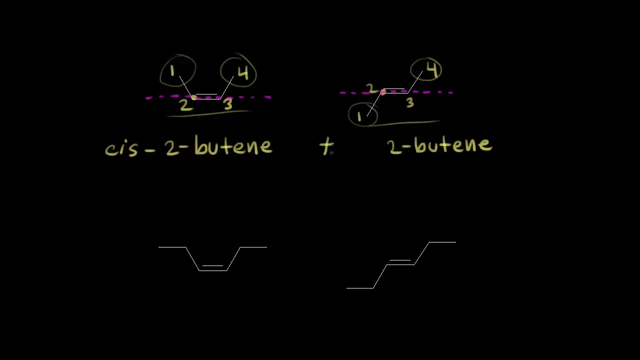 So this is the trans isomer. I'm going to write trans here in italics. attempt to anyway. So we have cis-2-butene and trans-2-butene. These are different molecules with different properties, If you want to use cis-trans terminology. 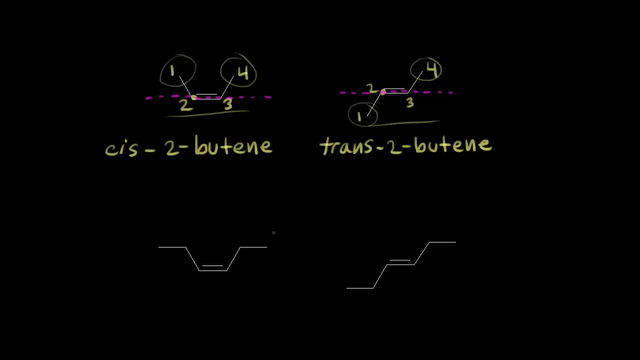 you're looking for two identical groups and you are comparing them. So let's look at these next two examples here and figure out which one is cis and which one is trans. We're looking for identical groups, So over here we have an ethyl group attached to our double bond. 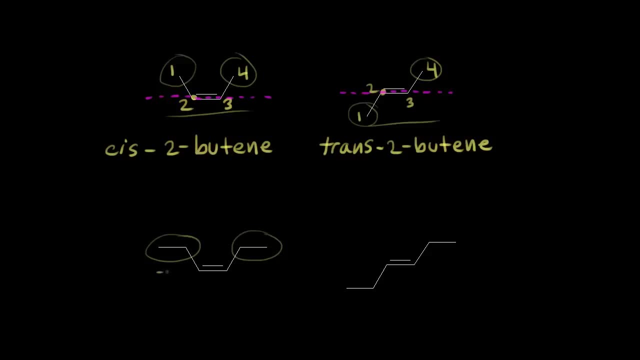 and on the right we have an ethyl group attached to our double bond. Those two ethyl groups are on the same side of our double bond, so this must be the cis isomer. On the right we have this ethyl group and this ethyl group are on opposite sides of our double bond. 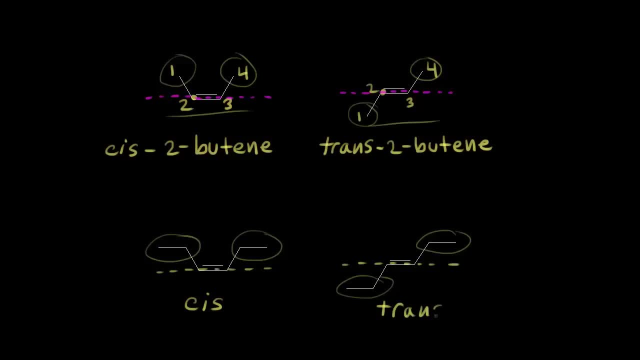 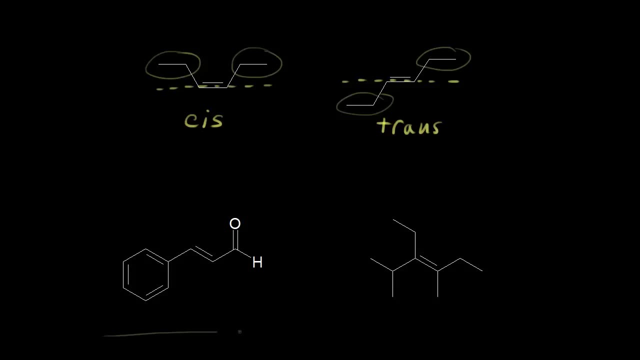 So that must be the trans isomer. Alright, let's do some more examples, So I'll go down to here. On the left we have the cinnamaldehyde molecule. We're looking for two identical groups so we can use cis or trans. 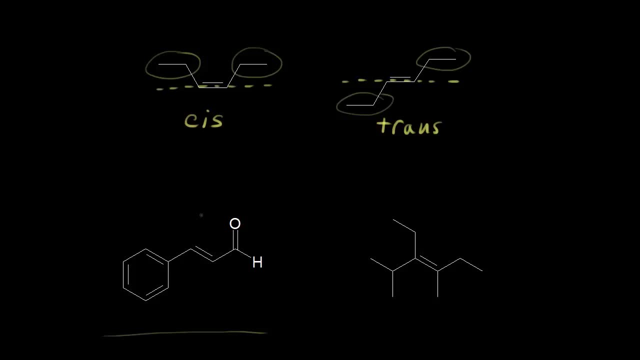 You can also use hydrogens. Right, You can use a methyl group or an ethyl group. So if we look at our double bond, we know there's a hydrogen attached to this carbon and we know there's a hydrogen attached to this carbon. 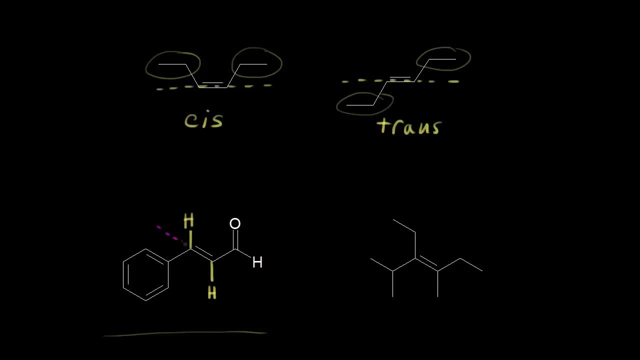 And those two hydrogens are on opposite sides of our double bond, So I'm drawing a line here to make it easier to see. Right, These two hydrogens are on opposite sides, So we're talking about trans here. Those hydrogens are across from each other. 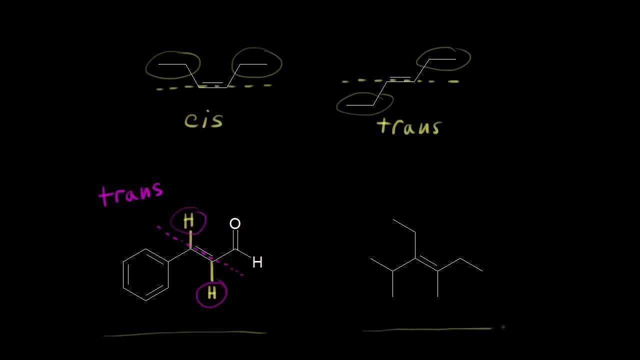 What about the tetrasubstituted alkene on the right? We need two identical groups to use our cis-trans, And here we have an ethyl group. and here we have an ethyl group. Right Over here we have a methyl group. 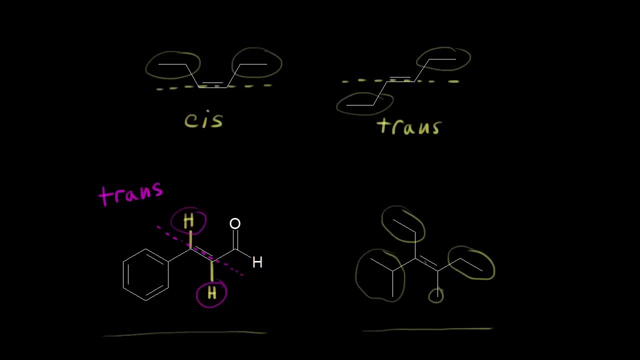 and an isopropyl group, But the two methyl groups are on the same side of our double bond. So I draw a line in here and we see that these two groups are on the same side. Therefore, we're talking about cis here. 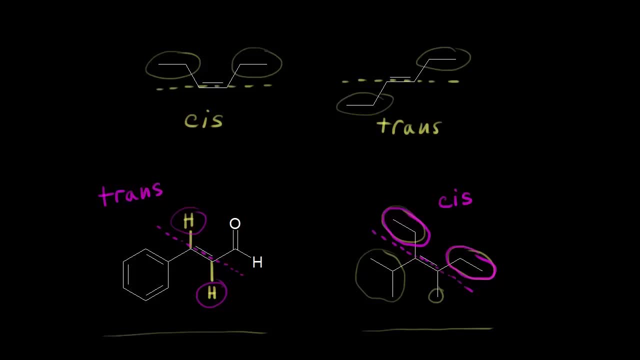 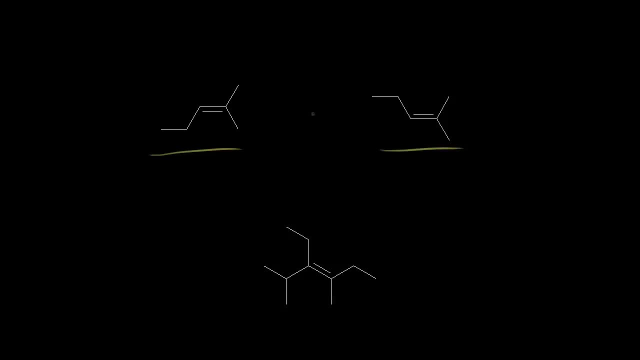 So this double bond has a cis configuration. Let's compare the drawing on the left to the drawing on the right. The first time you look at these two drawings you might think these are two isomers and I could use cis-trans terminology to distinguish between them. 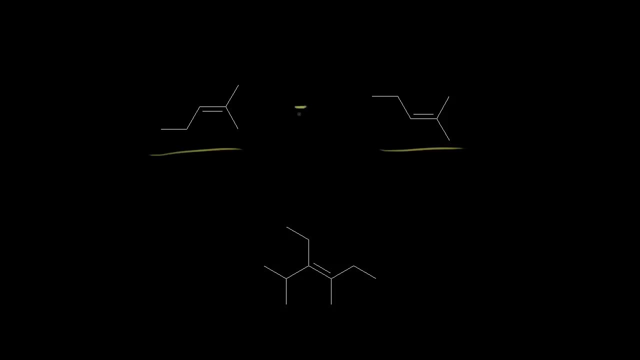 However, you can't, because these are just two ways to represent the same molecule. If you picked up this molecule on the left and you flipped it up, you would get the drawing on the right, So they're not isomers of each other. 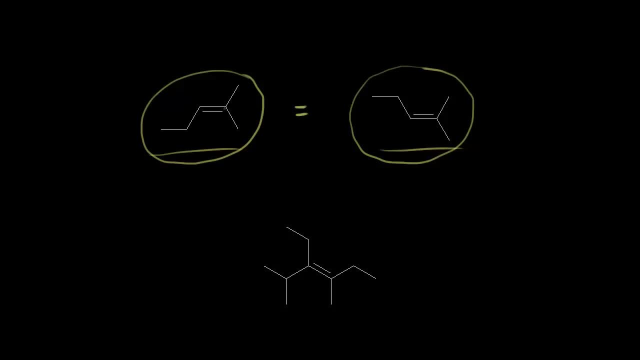 It is the same molecule And a fast way to figure that out is to look at this carbon And you can see you have two identical groups bonded to that carbon, So you can't use cis-trans terminology That's different from the example we did a minute ago. 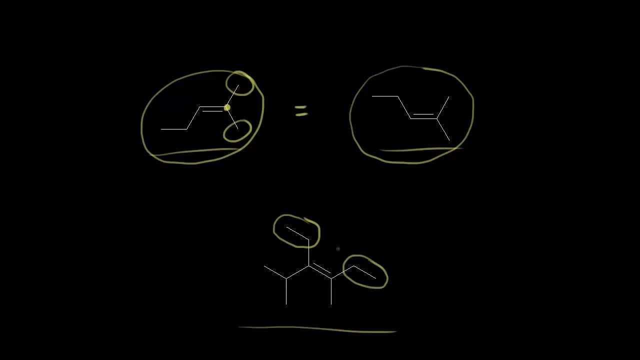 We had two identical groups, these two ethyl groups, here. However, those two ethyl groups weren't bonded to the same carbon. Those two ethyl groups are bonded to different carbons. This ethyl group is bonded to this carbon and this ethyl group is bonded to this carbon.